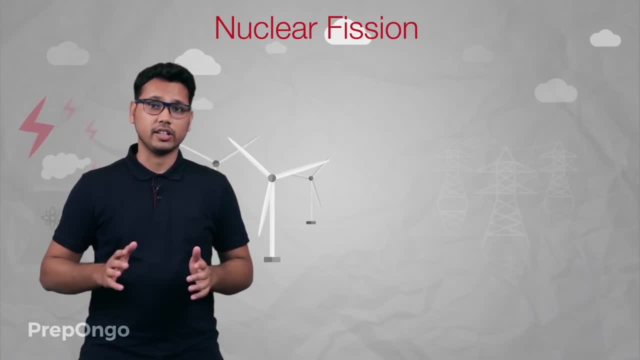 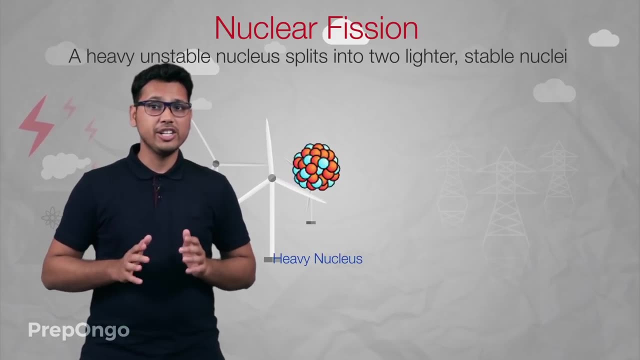 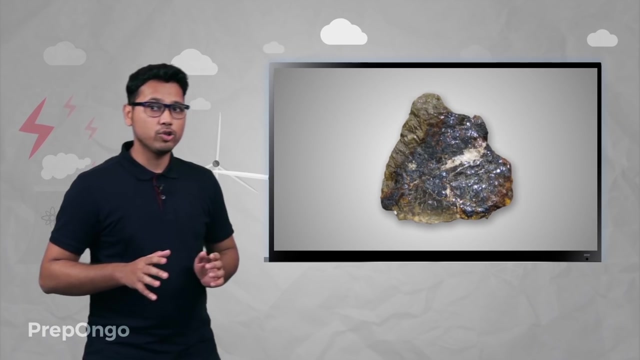 splitting of some bigger thing into some smaller thing. Now in nuclear fission, a nucleus of a heavy, unstable nucleus splits into two lighter and stable nuclei. Now if we zoom in into the heavier elements, like uranium and plutonium, we'll find out that their nucleus 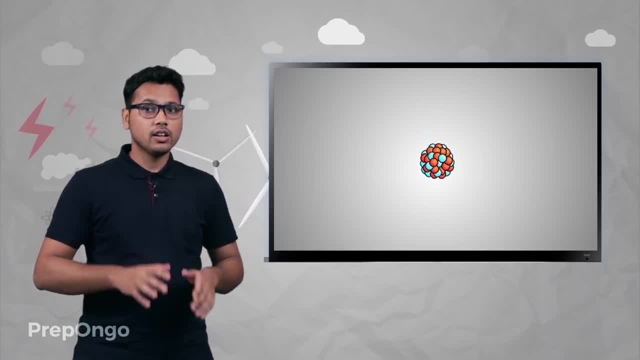 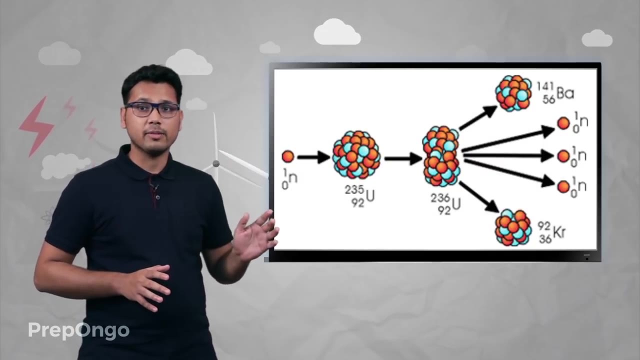 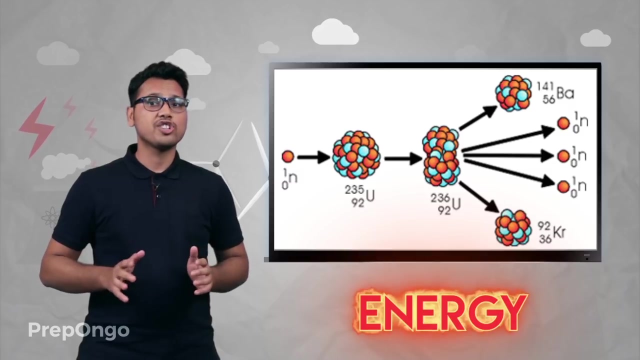 is highly unstable. So when a slow-moving neutron is bombarded onto these elements, the nucleus absorb that neutron and then it splits into two lighter nuclei of barium and krypton. Now these two nuclei are stable in nature and a huge amount of energy is released in this process. 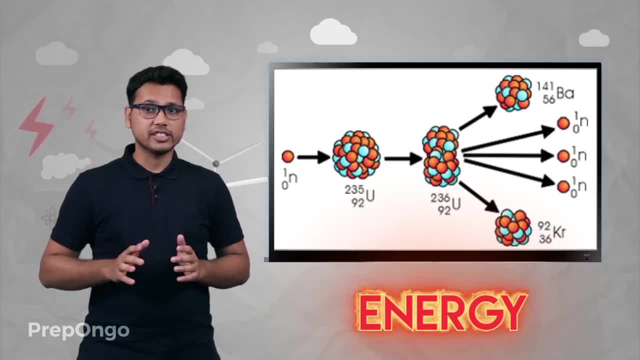 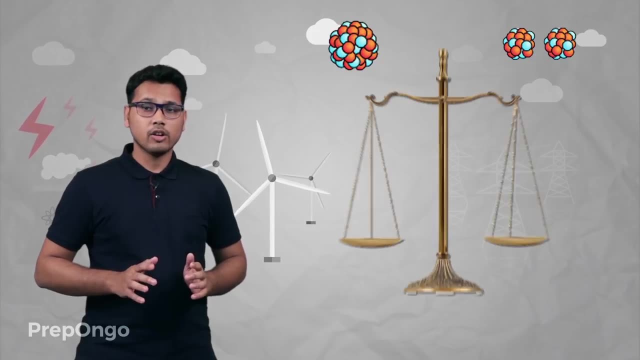 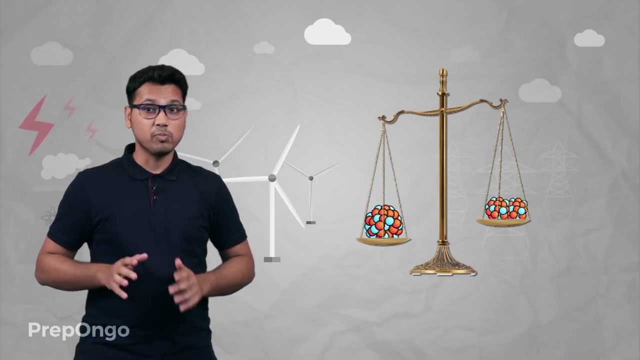 Since this process involved the breaking of a heavy nucleus into two nuclei, hence it is termed as nuclear fission. Now, in this process, where does this energy is coming from? Now, if you weigh the two lighter nuclei, you will find out that their weight will be a little smaller. 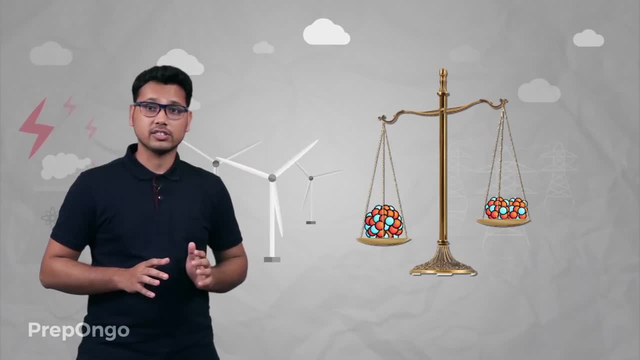 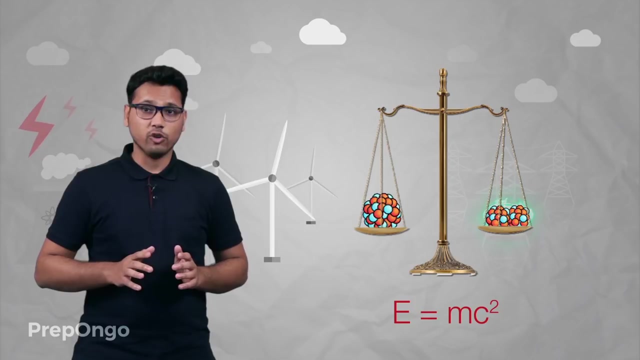 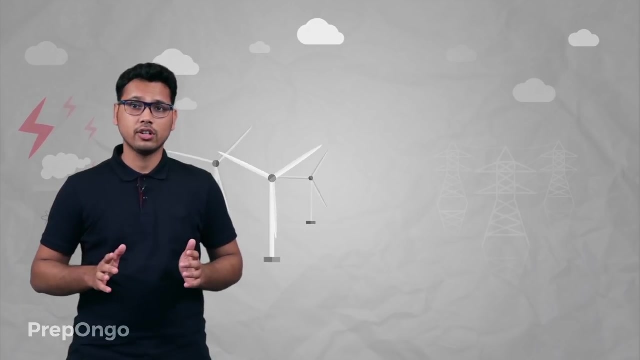 than the weight of this heavy nucleus. So we can say that that mass which is lost is converted into this huge amount of energy by using Einstein mass-energy equivalence- that was E- is equals to NC square. Now the energy produced in this process is really huge: One gram of. 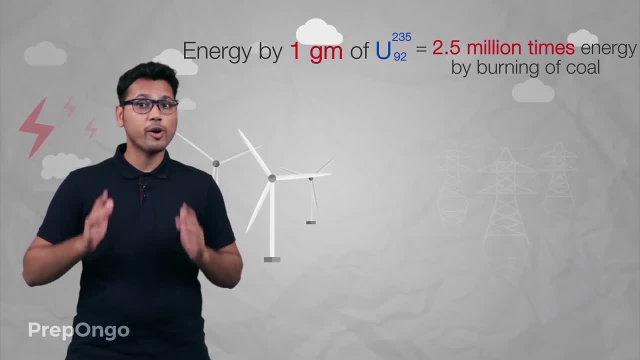 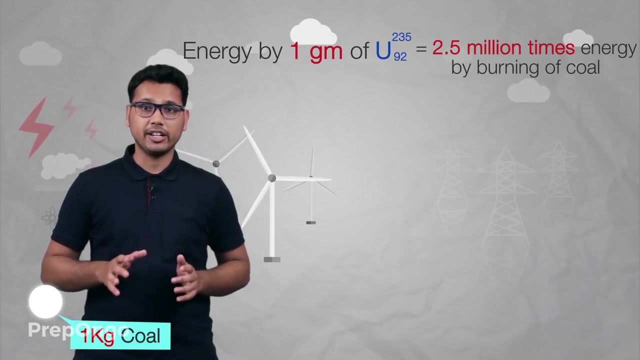 uranium-235 produces around 2.5 million times the energy produced by one gram of coal While burning. Now, to understand this scale, consider that burning of one kg coal is represented by this dot. Now, if we have to express the energy released by one gram of uranium in terms of this, 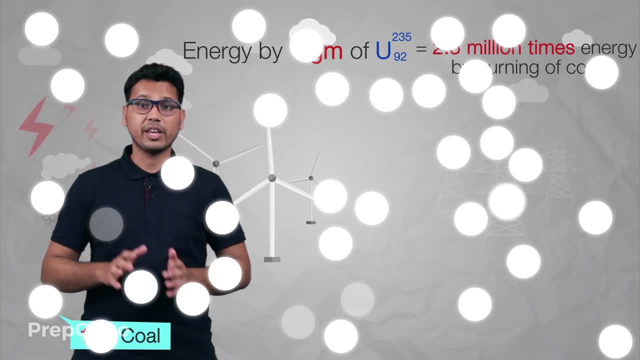 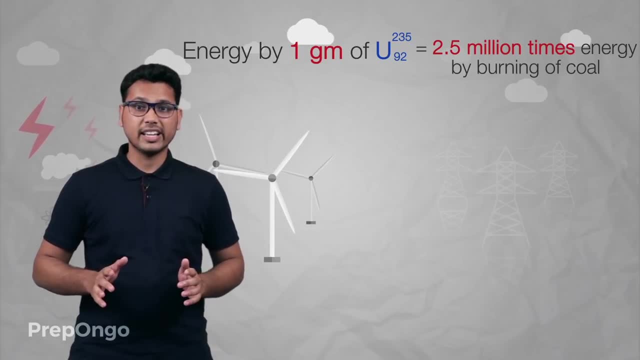 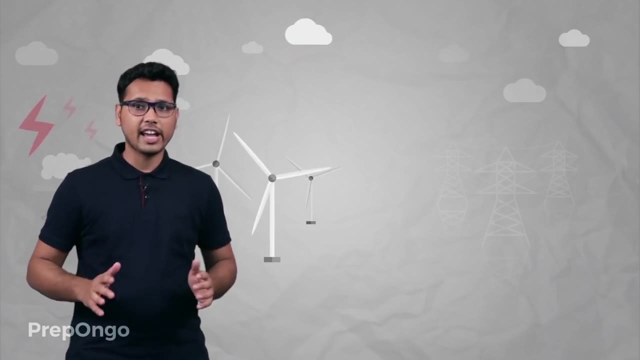 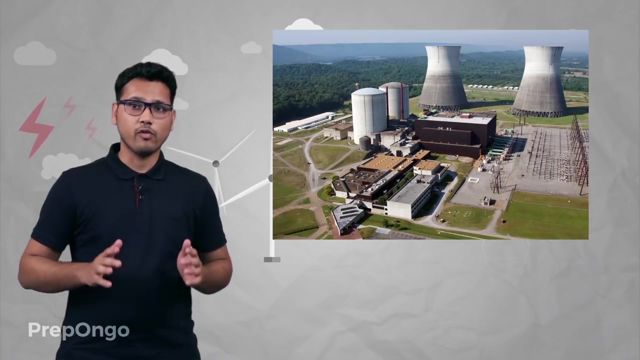 dot. our whole screen will be covered by these dots, So we can say that the energy produced by uranium is really huge in comparison to coal or petroleum. The energy from the nuclear reactions can be used in a controlled manner in nuclear reactors to produce steam from water and. 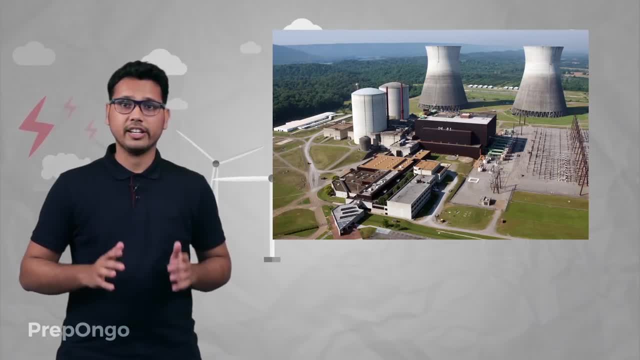 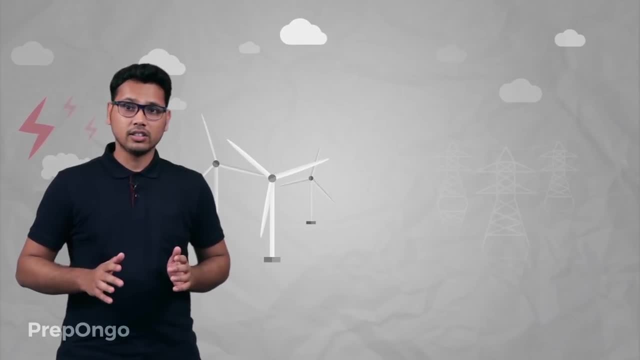 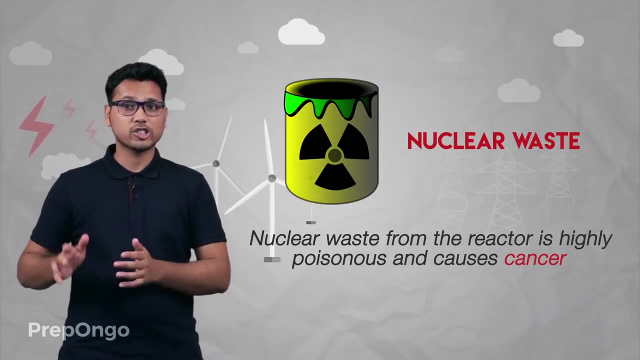 then this steam can be used to run the turbines to get electricity. Now the major problem that arises in the use of nuclear reactors is that the waste which is left out after the nuclear reactions is highly poisonous and it also causes cancer. So we have to dispose of this waste in a very far away places from the 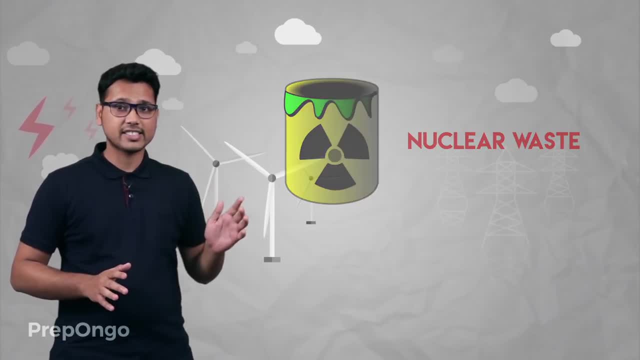 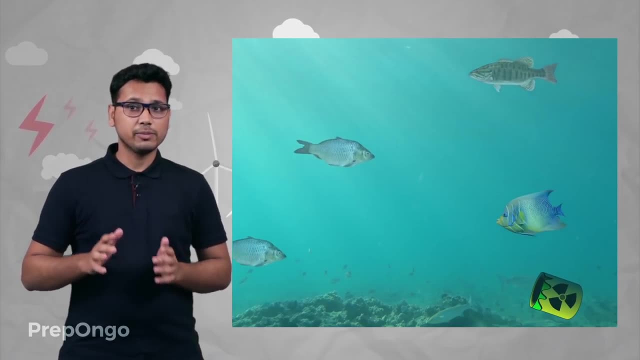 community. So the disposal of the waste from the nuclear power plant are done in deep sea so as to avoid possible contact with them. But ultimately this waste can be used in a controlled manner. by using nuclear reactors to produce steam, waste cause damage to the aquatic life. Also, the nuclear power plant should be operated very safely. 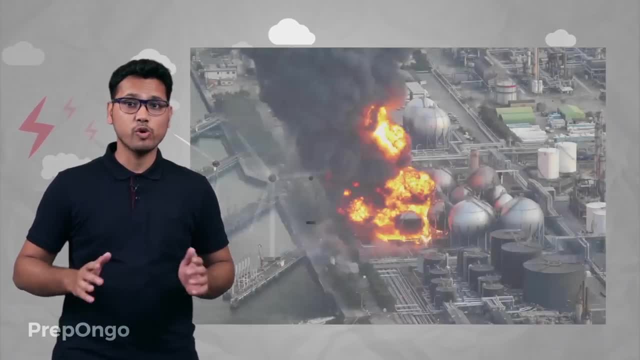 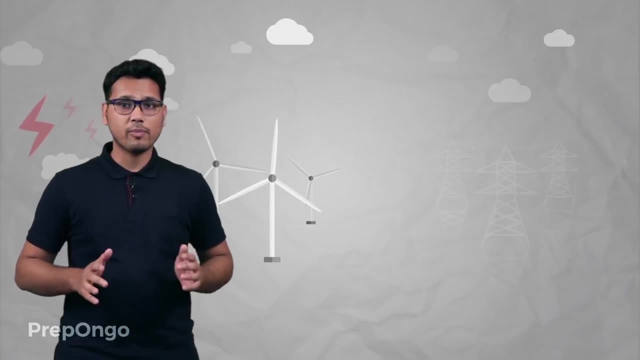 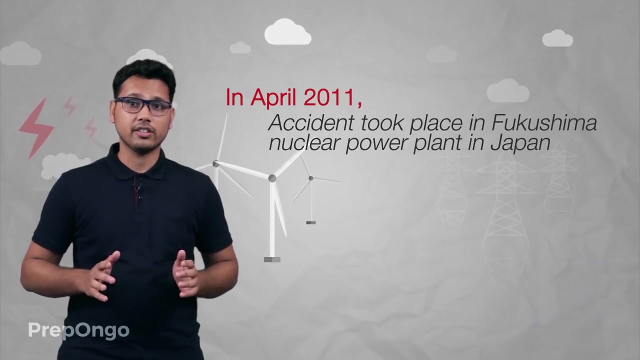 as a slight error can result in explosion and spread out of the radioactive nuclear waste into the surrounding. The recent nuclear power plant accident took place in Fukushima Daiichi in Japan in April 2011.. The good thing about this accident was that the casualties in this accident were. 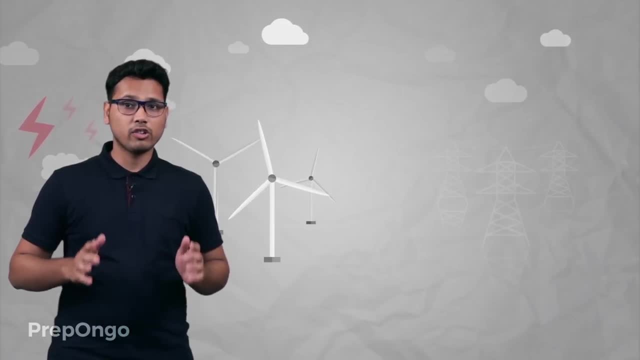 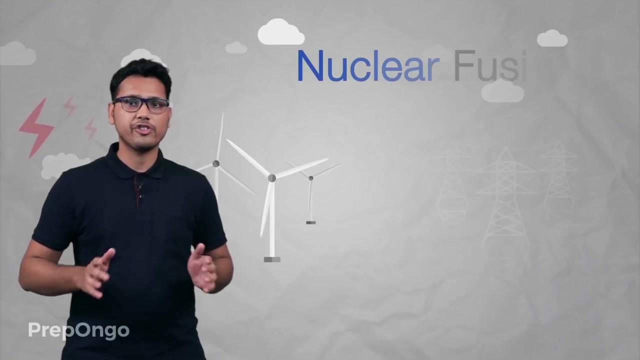 minimum. So if we somehow make the nuclear power plant safer and if we somehow find out a way to dispose of their waste, then nuclear energy can power up the world. So this was all about nuclear fission. Let's talk about nuclear fission now. Now, this is the process, which involves. 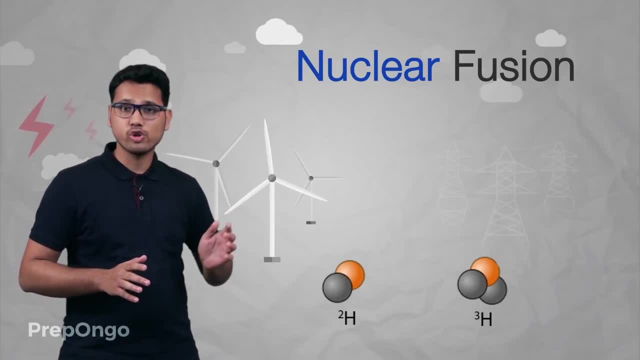 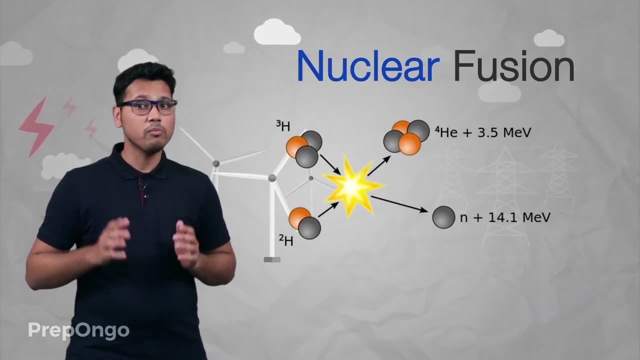 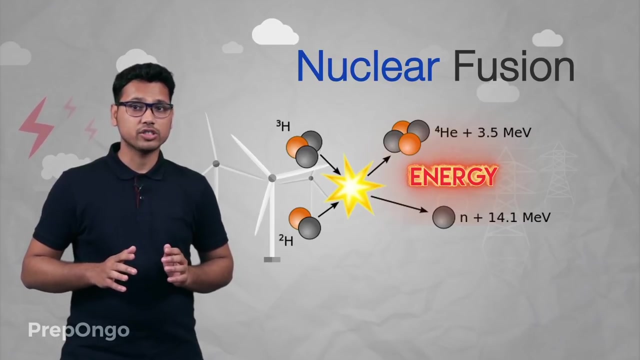 fusion of two lighter nuclei like hydrogen into a heavier nucleus like helium. Now in this process also a small mass is lost and that mass is converted into huge amount of energy. So we can say that in process of fusion also we get a huge amount of energy. There is one problem with fusion. 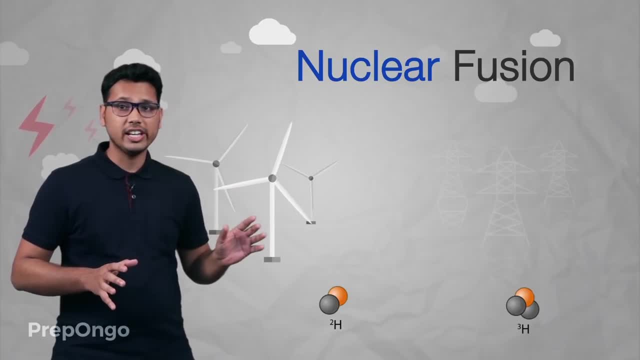 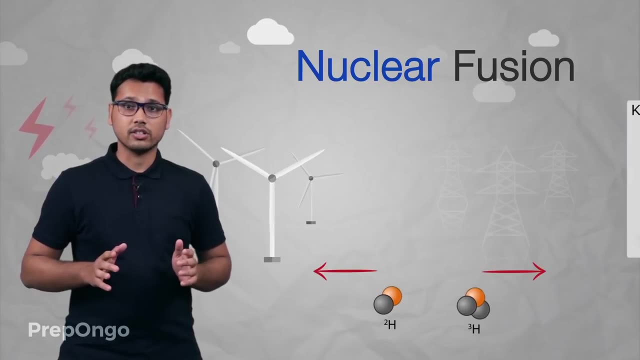 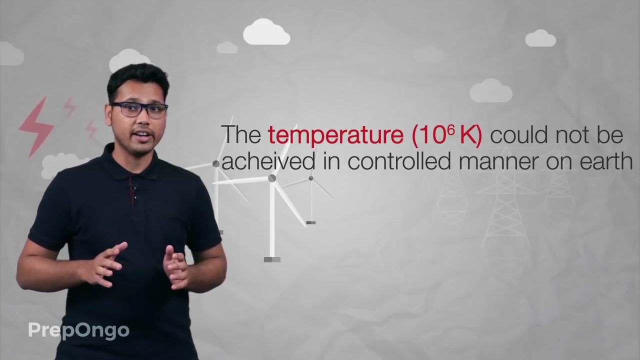 When we try to bring these two nucleus together, they experience a large amount of electrostatic repulsion. And now to overcome that repulsion we need very high temperatures. The temperatures up to 10 raise to power 6 Kelvin and those temperatures could not be achieved in controlled manner on earth. But if we look at Sun, the